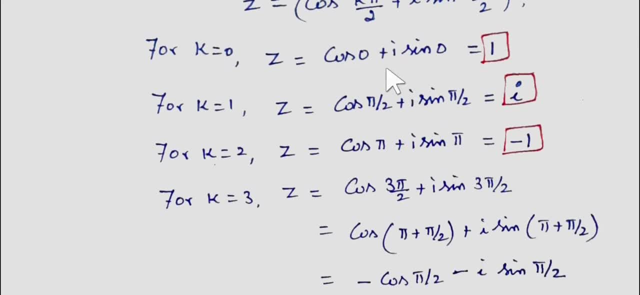 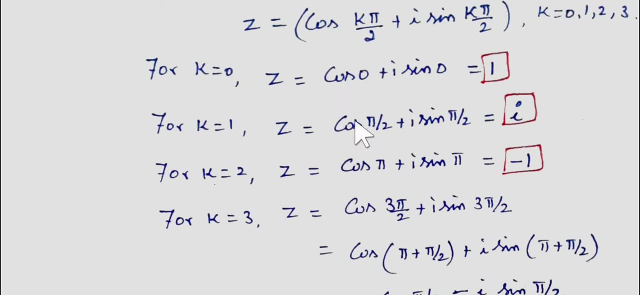 cos 0 plus i sine 0.. equal to 1 and for k equal to 1. if we substitute k equal to 1 here, then z is equal to cos pi by 2 plus i sine pi by 2, which is equal to i. If k equal to 2, then 2, 2 get cancelled, then we will. 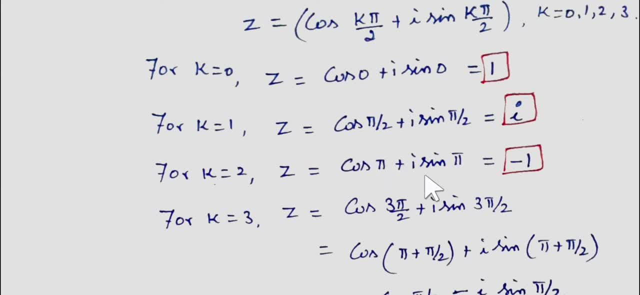 get cos pi plus i sine pi. Value of cos pi is 1 and sine pi is sorry. value of cos pi is minus 1 and the value of sine pi is 0. Then, for k equal to 3, we get 3 pi by 2.. 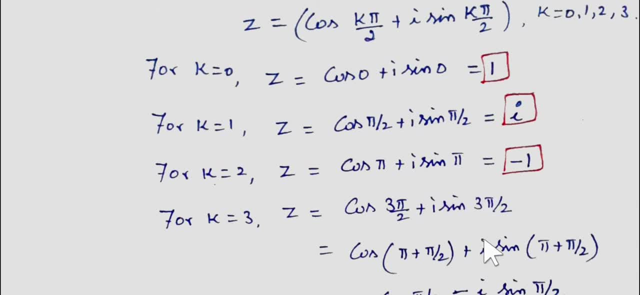 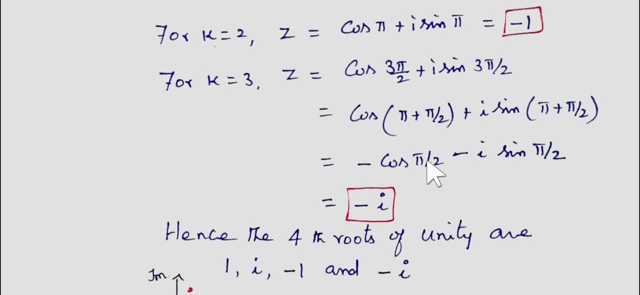 So cos, 3 pi by 2 plus i sine 3 pi by 2.. Now 3 pi by 2 can be splitted as pi plus pi by 2.. Anyway, pi plus pi by 2 present in the third quadrant. In third quadrant both cos and sine. 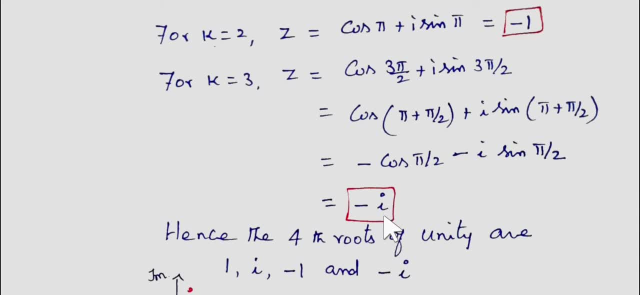 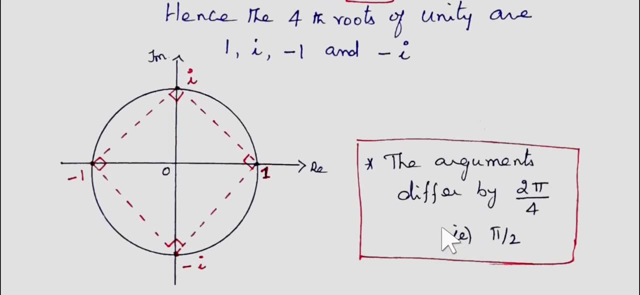 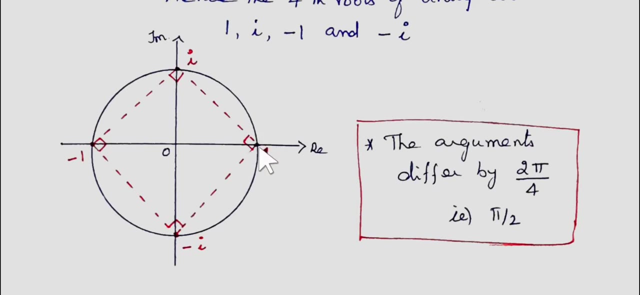 are negative, So we will get the value as minus i. Hence the fourth roots of unity are 1- i minus 1 and minus i, 1 i minus 1 and minus i. Now let us see the diagram. So we will get the kinetic representation of fourth roots of unity: 1, and this is i, then minus 1.. 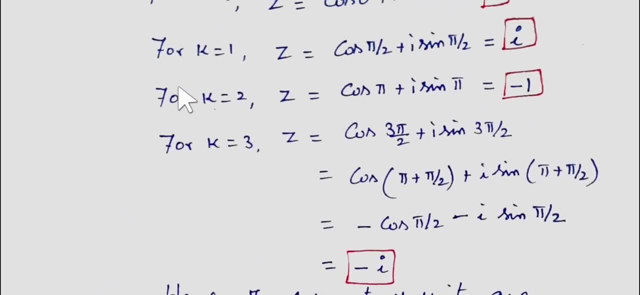 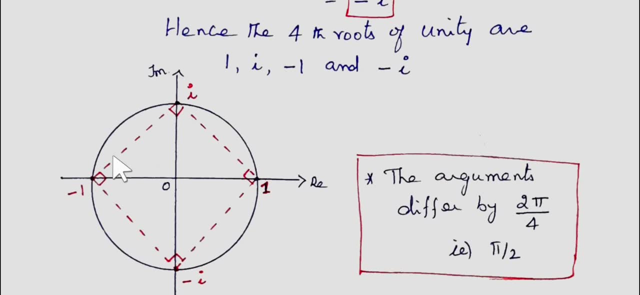 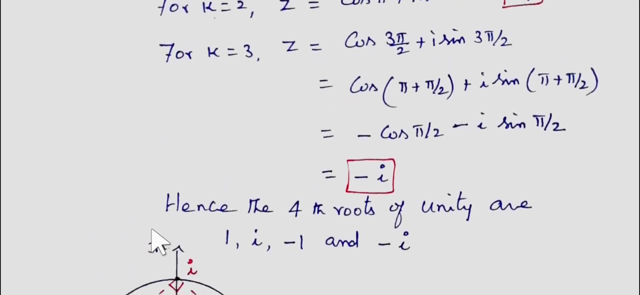 That is, i means 90 degree Cos pi by 2 plus i sine pi by 2.. So the second root will come here and the third root after pi by 2, rotation: cos pi plus i sine pi, that is minus 1.. And the fourth root is cos 3 pi by 2.. So 3 times pi by 2.. So 1, 2 and 3 times pi by 2 means it will. 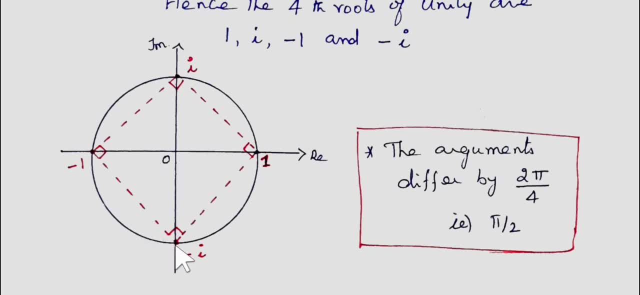 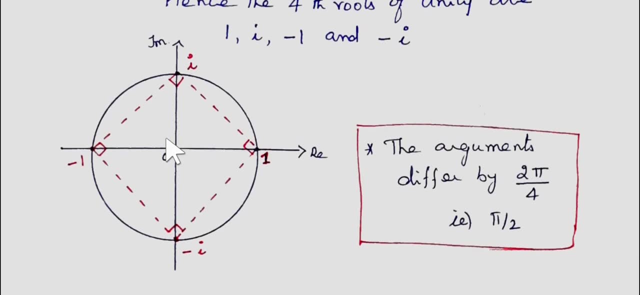 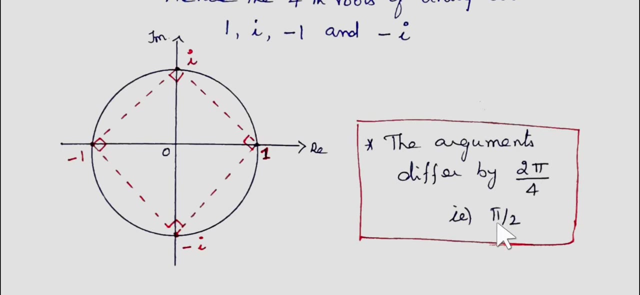 1, 2 and 3 times pi by 2 means it will come here. come here that is minus i. if we join all the fourth roots of unity, we get a square. here the arguments differ by 2, pi by n, that is, n is equal to 4. so 2 pi by 4, pi by 2. here the arguments. 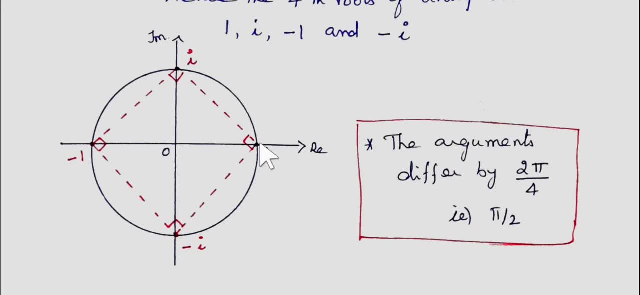 differ by pi by 2. so after pi by 2 rotation, the second root will come. so from here, after 190 degree rotation, the third root and likewise the fourth root will come. now the fourth roots of unity are 1 i minus 1 and minus i.